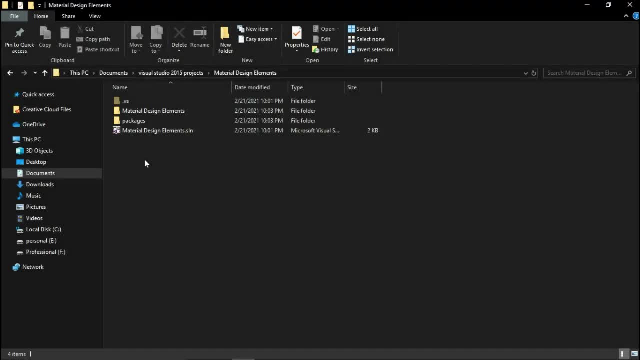 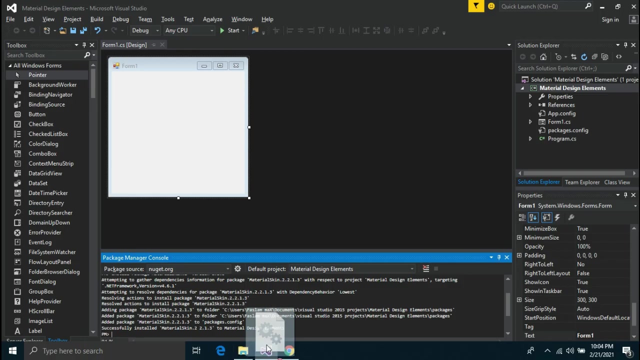 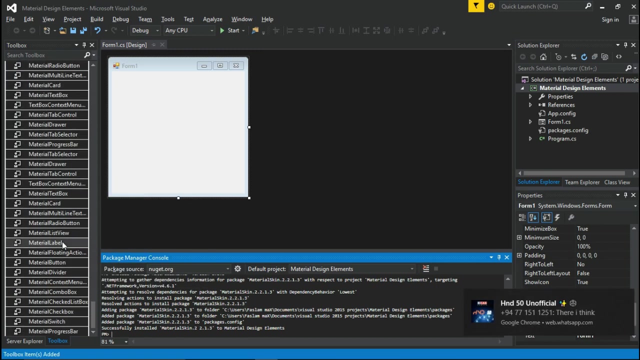 you will see a successfully installed. then go to file where you save the project and follow the path packages: materialskin.2.2.1.3- lib- net461 and drag materialskindll file to your Visual Studio's toolbox. now you can see the additional material components in the toolbox. 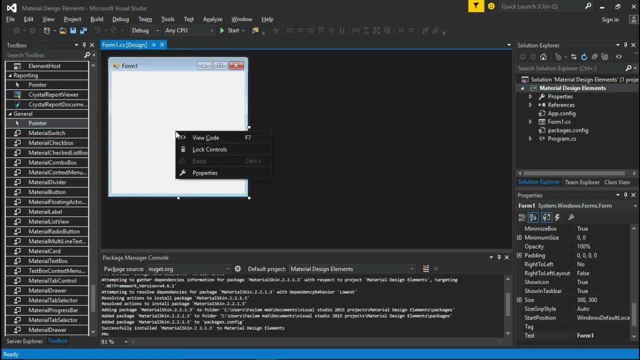 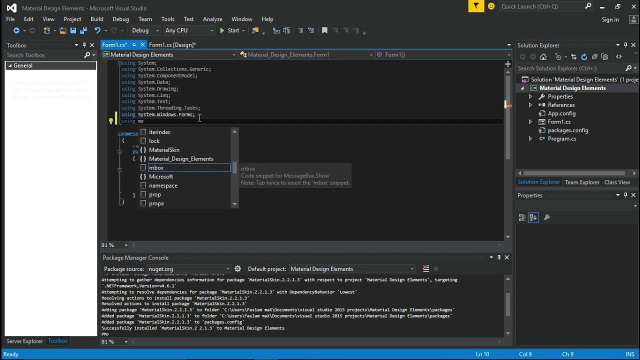 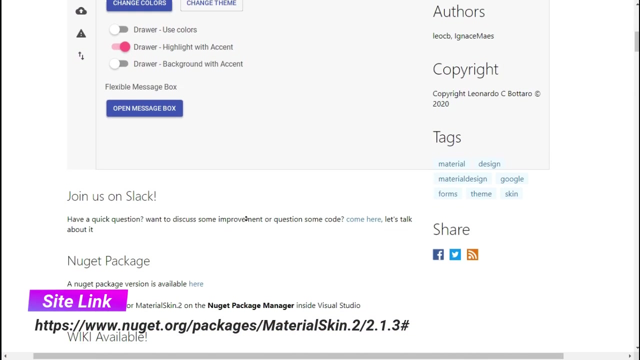 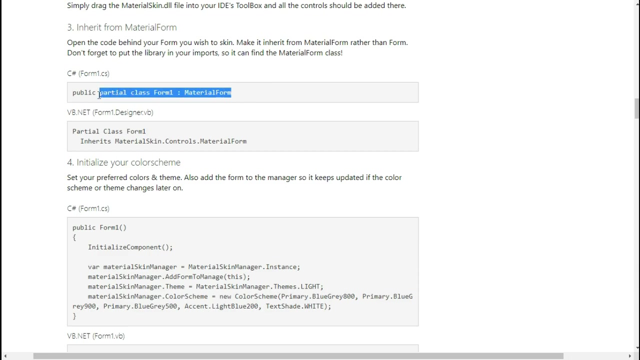 now let's change the form style to material form design. for that, right click the form and view code. add this lines of code at the top of your code. now go to the material skin site link given in the description. scroll all the way down until you see this code. copy the code and come back to Visual Studio and replace it with the this: 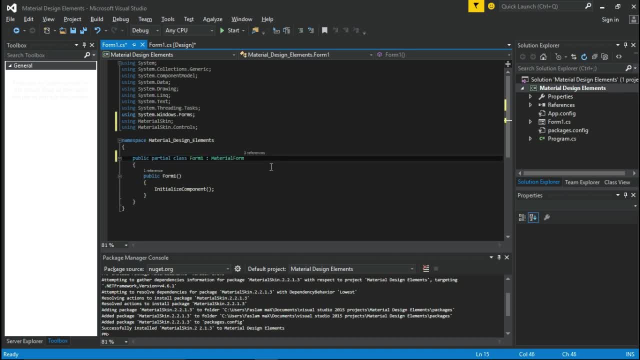 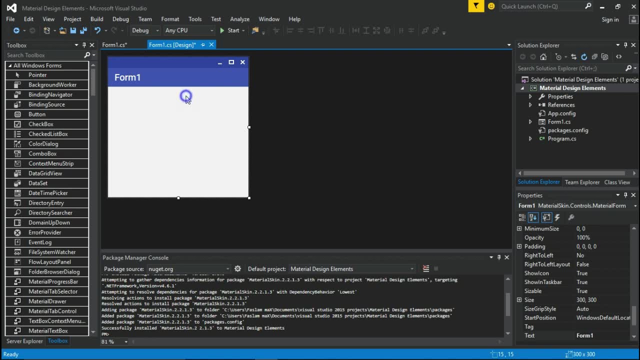 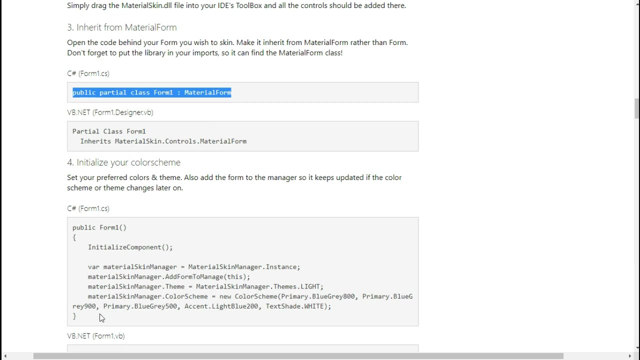 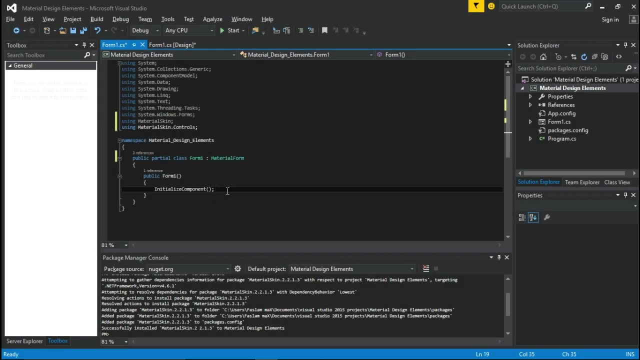 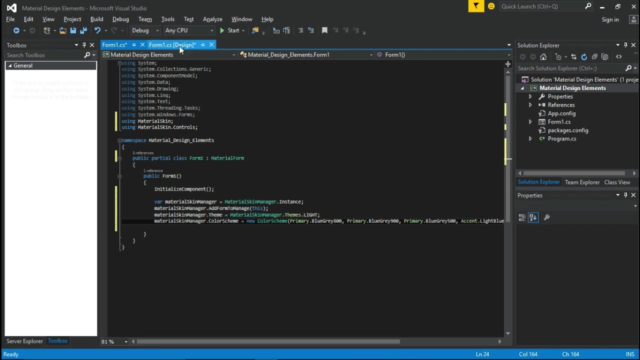 now, if I go to the forms design view, you can see how the stock form changed to a material form design. go back to the code. then navigate to material skins site and copy this lines of codes and paste it inside the initialize components. Now you are all done. 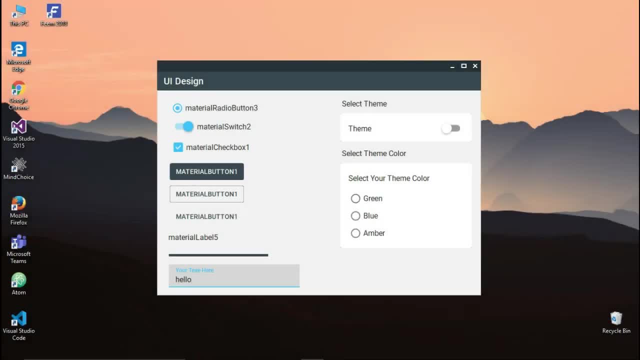 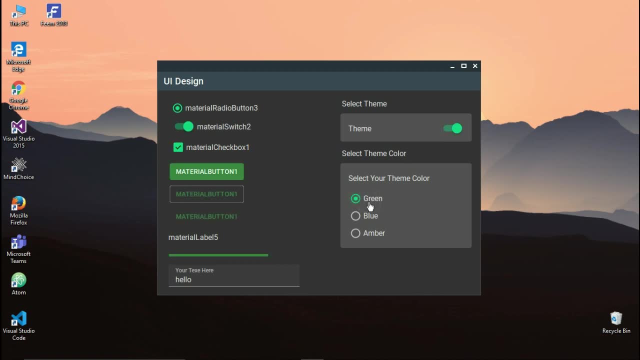 Now you can work with this material components. In the next video, I will show you how to make a dark and light theme toggle in your windows form And also how to change the secondary color scheme of your windows form. If the video is useful, a sub to the channel would be appreciated and I will catch you. 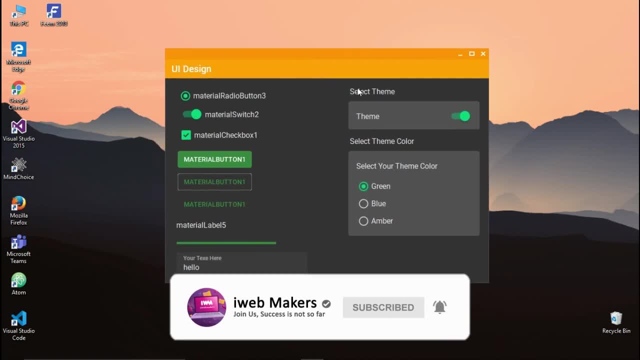 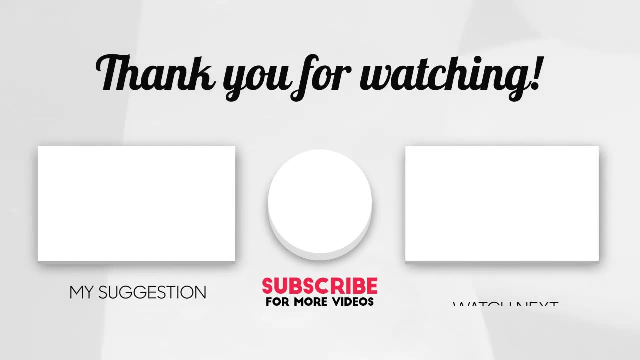 guys in the next one.